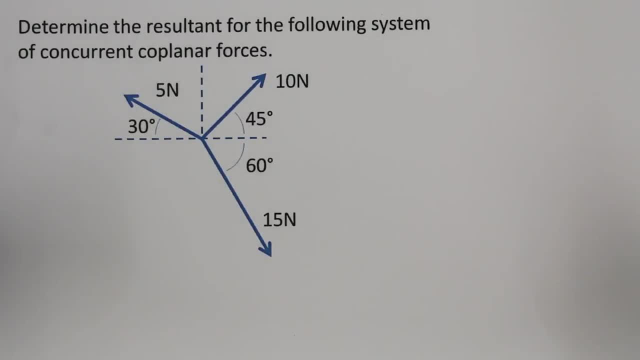 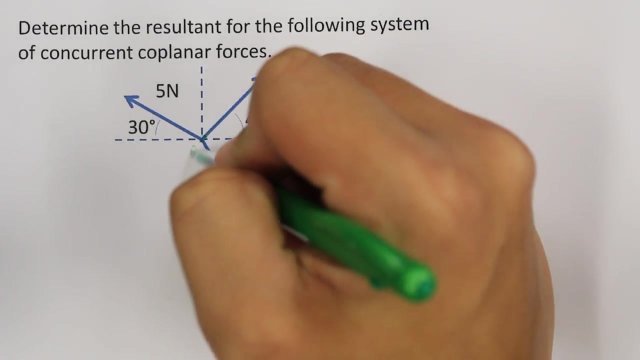 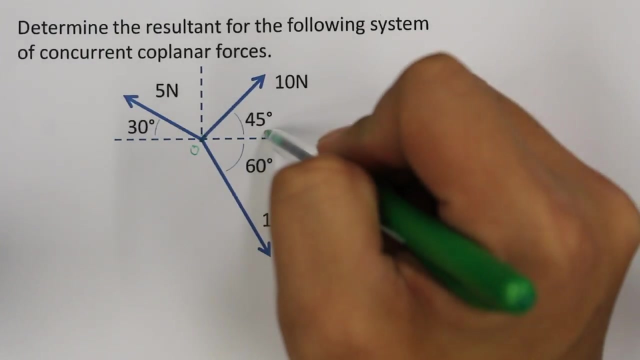 Hi guys, this is an example for calculating the resultant force for a concurrent coplanar system of forces. So what we have here is three forces that are seen to act at one single point. We could call that point O and we see a 10 Newton force at 45 degrees from the horizontal, If this was the x-axis, and 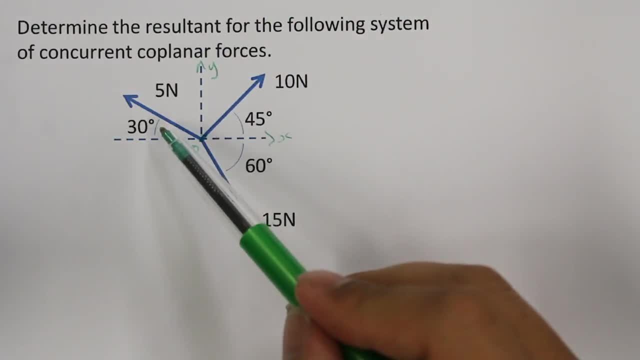 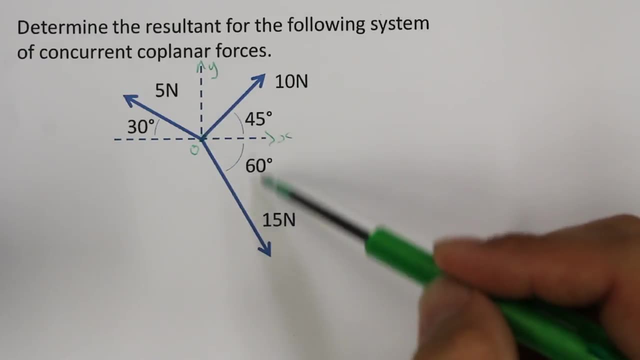 this is the y-axis. we have a 5 Newton force acting 30 degrees from the negative x-axis and a 15 Newton force acting at an angle of 60 degrees from the positive x-axis. The forces which we have here can be resolved into their x. 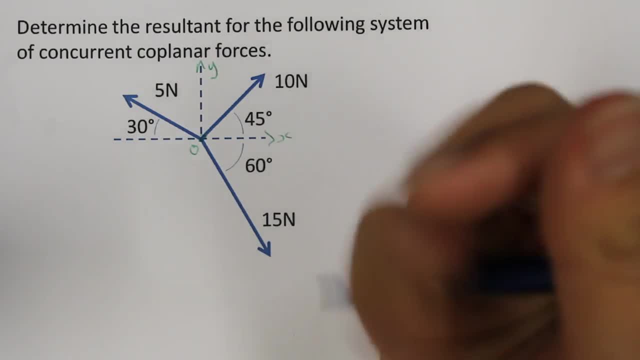 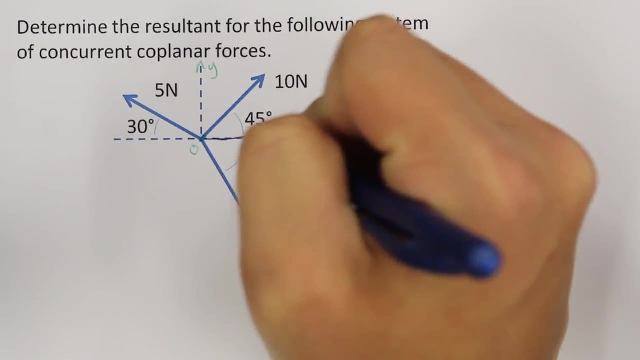 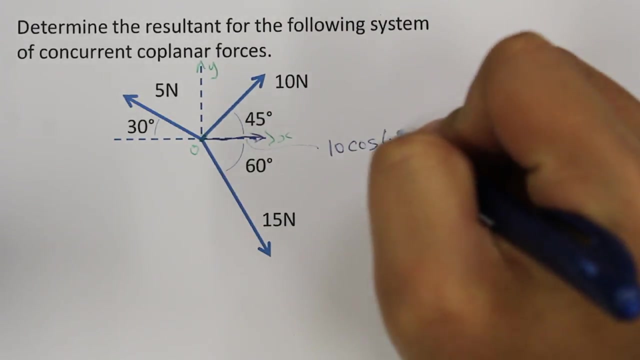 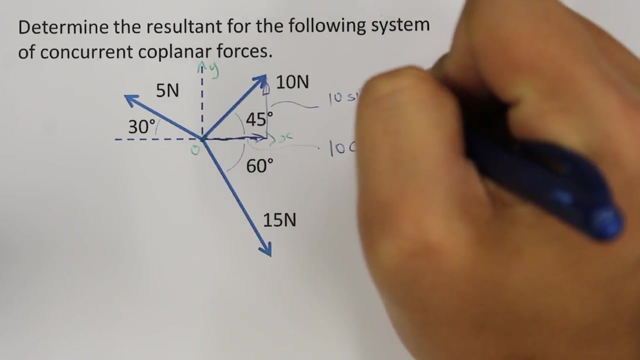 component and y component. So, for example, the 10 Newton force can be replaced by a force going towards the right, where its magnitude would become 10 cosine 45, and a y component which would become 10 sine 45. Also for the 5 Newton force, that 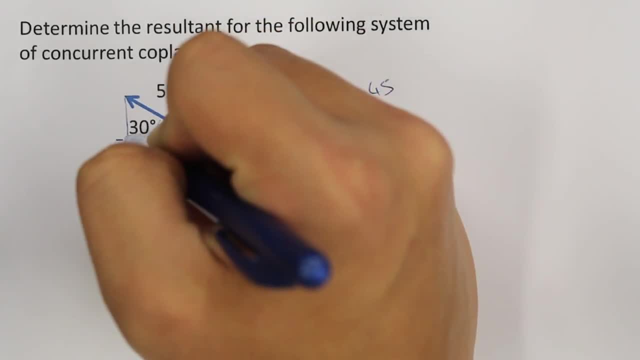 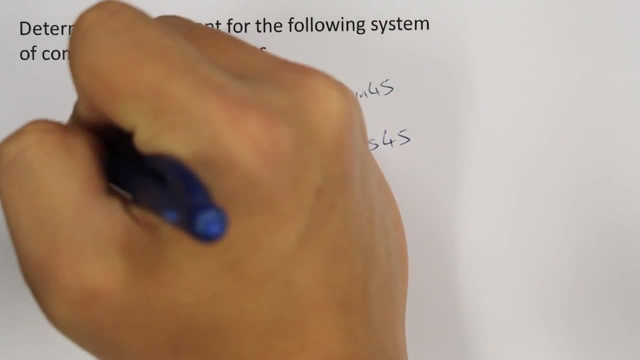 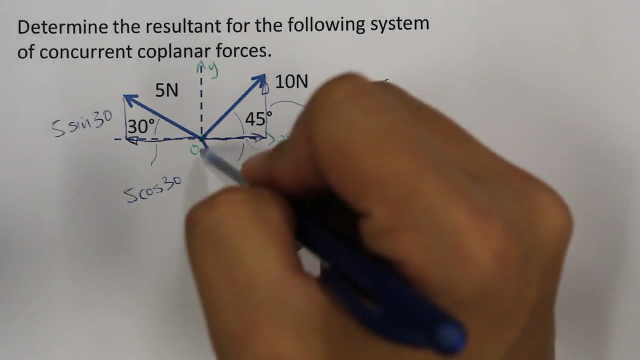 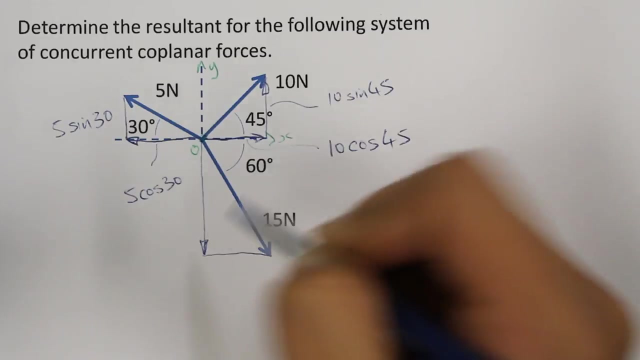 can also be resolved into a component in the x direction, which will be 5 cosine 45.. 30 and 5 sine 30. as we see here, The 15 Newton force can be resolved into a y component and the x component- The y one is pointing downwards. This will become: 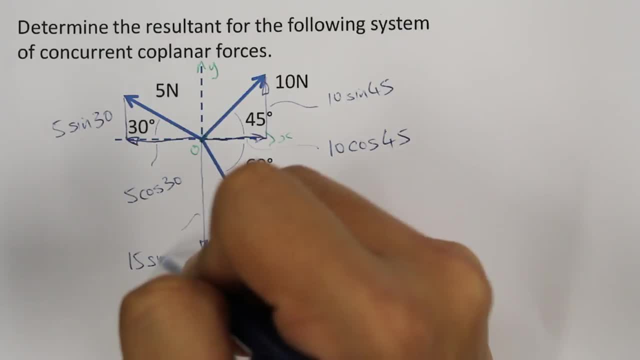 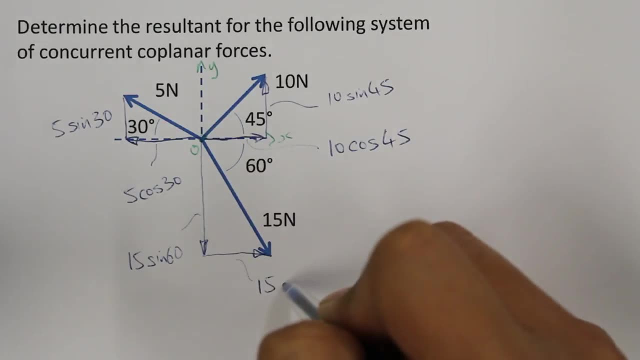 15 sine 60, and this component here would become 15 cosine 60.. If you need a review of these finding force components, there will be a video made available. Just click on the link that will show soon. Alright, now the first step for finding the resultant is to find the components of each. 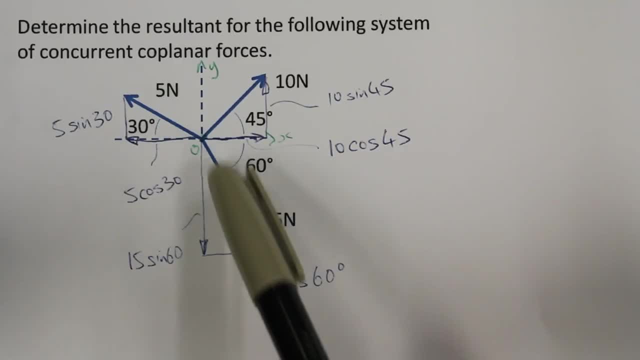 force, and we can see x components for each vector and y components for each vector. We'll go through the tabular method for finding the resultant Alright, so we'll construct a table. In this table we'll have the description. We'll have 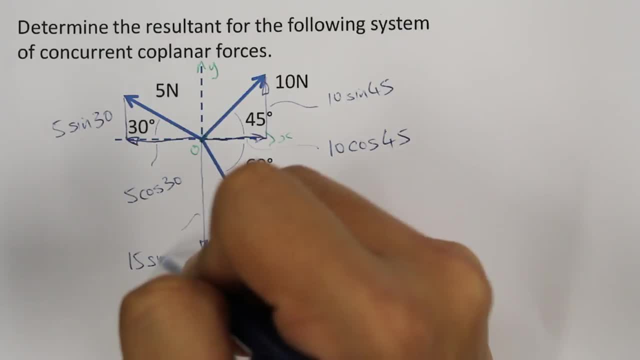 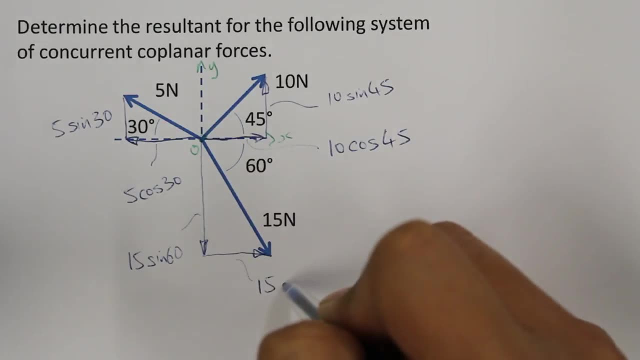 15 sine 60, and this component here would become 15 cosine 60.. If you need a review of these finding force components, there will be a video made available. Just click on the link that will show soon. Alright, now the first step for finding the resultant is to find the components of each. 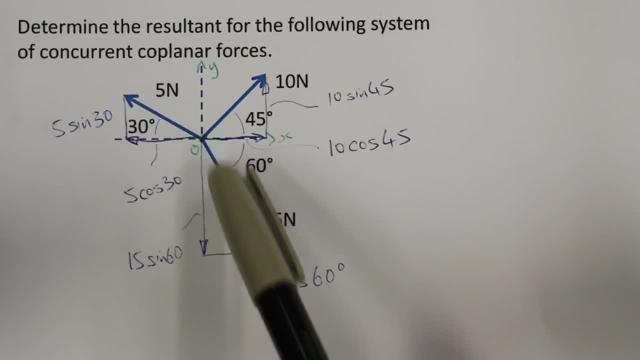 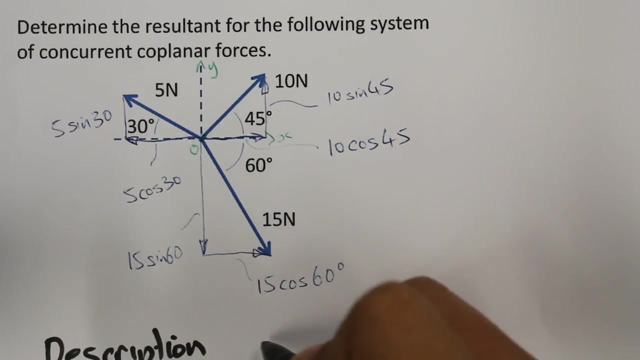 force and we can see x components for each vector and y components for each vector. We'll go through the tabular method for finding the resultant OK, so we'll construct a table. In this table we'll have the description, We'll have the 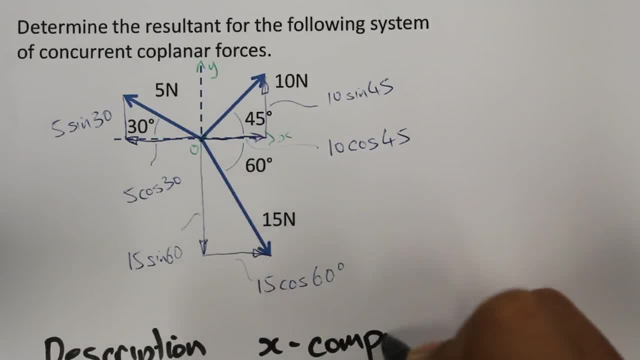 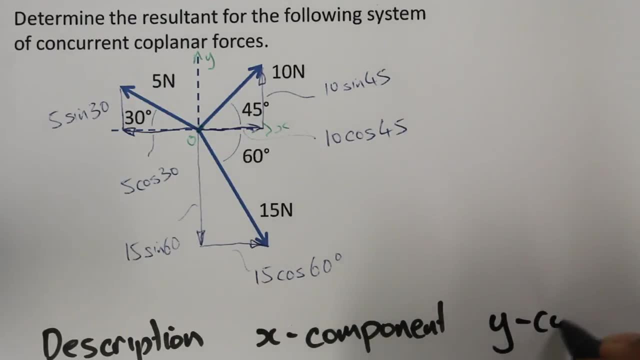 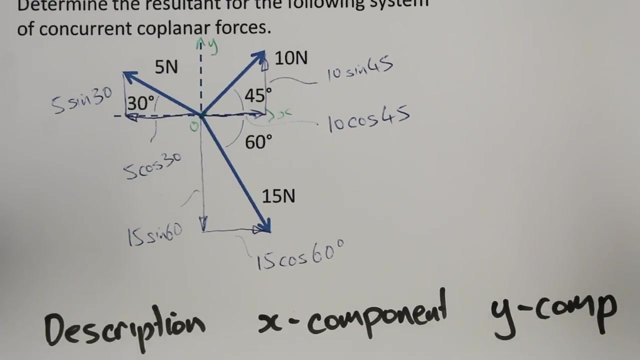 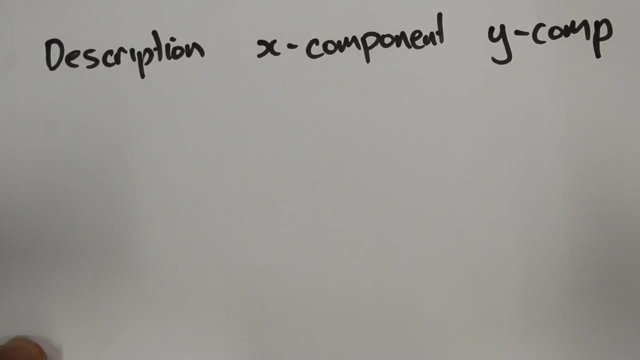 x component And also the y component. All right, so the description would be X and Y. we have those three forces there and we'll write them. I'm just going to write them down here, So I'll just move this up. Our first force was a 10. 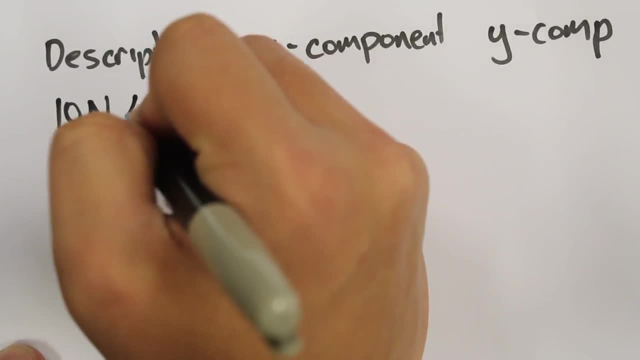 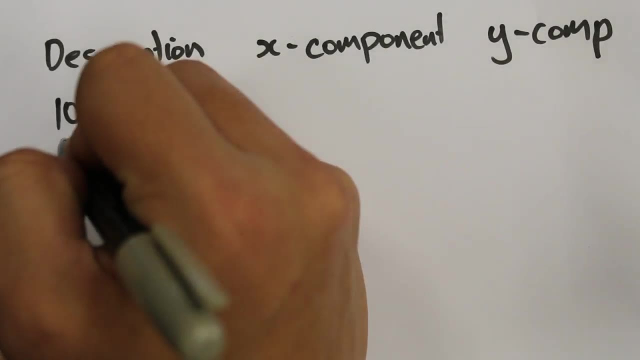 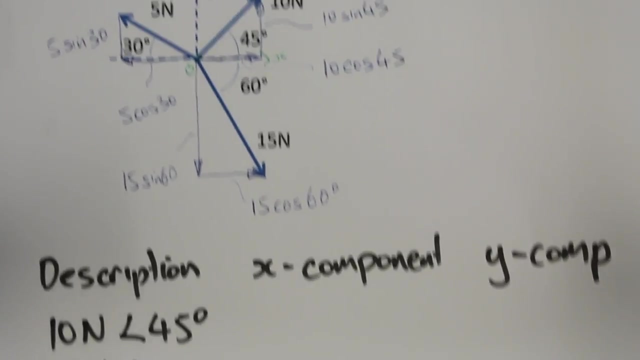 Newton force. It was acting at an angle of 45 degrees as measured from the x-axis. We also have a 5 Newton force which was acting at an angle of 150 degrees. So if we look here, the angle measurement from here to this point here will be: 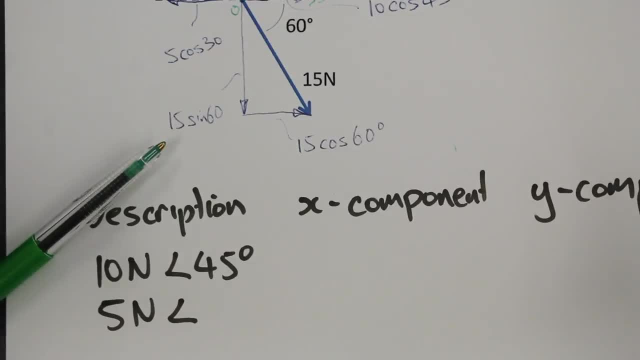 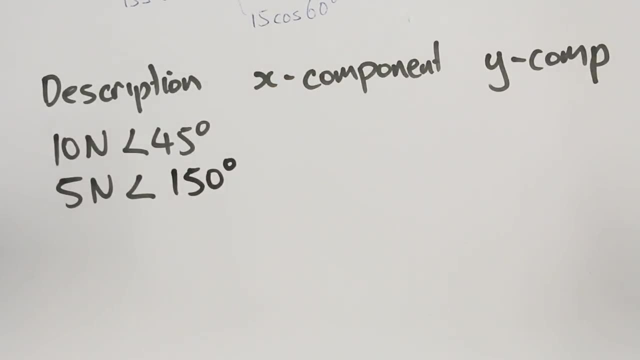 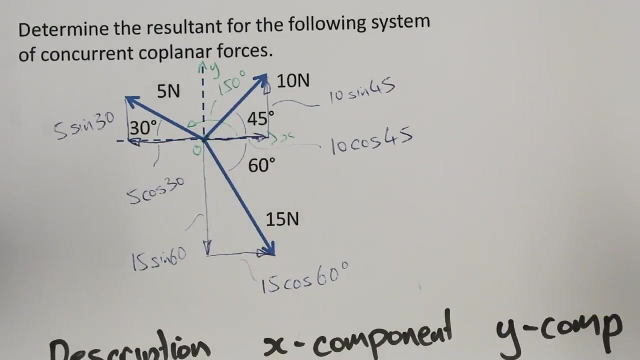 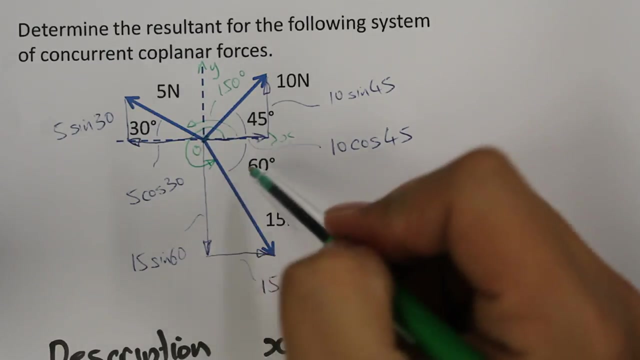 150 degrees. So here our measure is 150 degrees, Same for our 15 Newton force. So if we look at this again, the measure of angle going from the x-axis all the way around to our vector, there will be 360 minus 60 or 300. 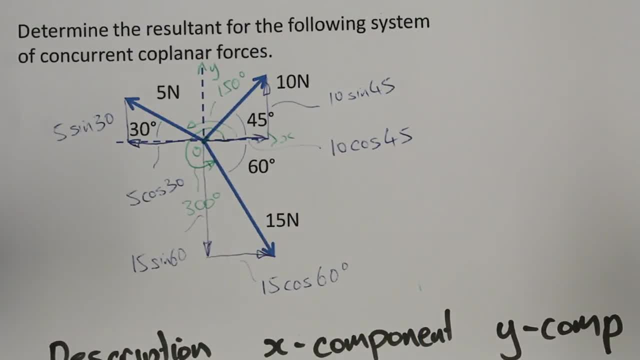 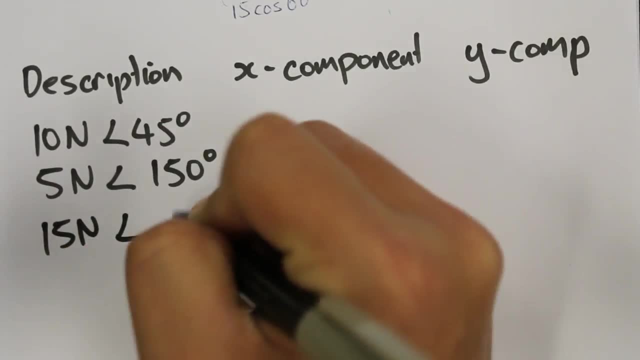 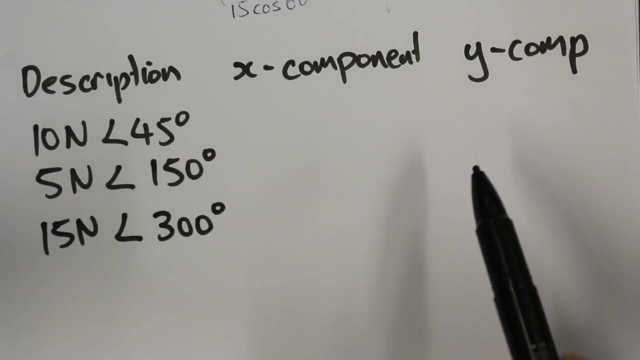 degrees. So let's write that component down. So the 15 Newton force is at an angle of 300 degrees. Alright, so we can write down the x component and y component for each force, as long as we measure the angle as measured from the x-axis. 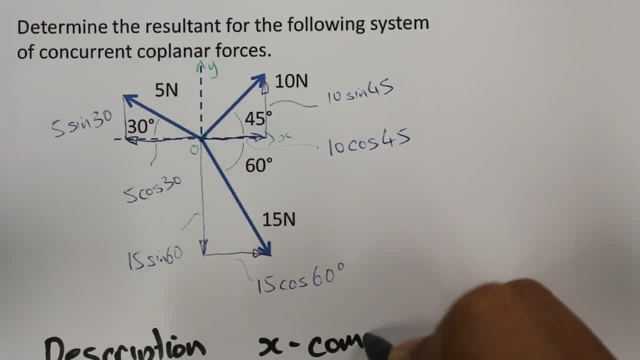 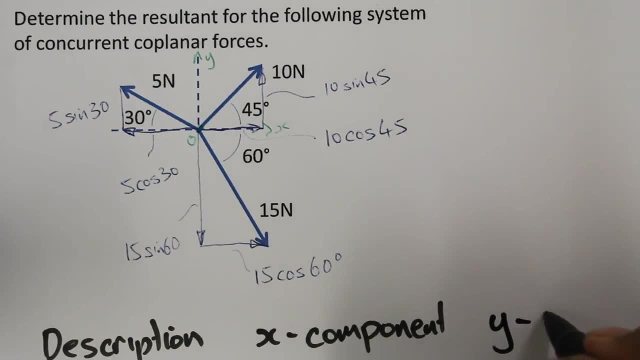 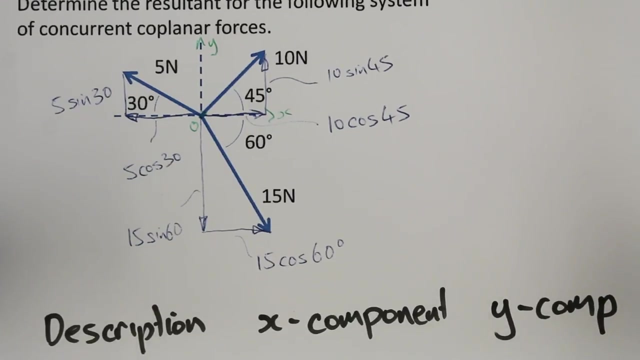 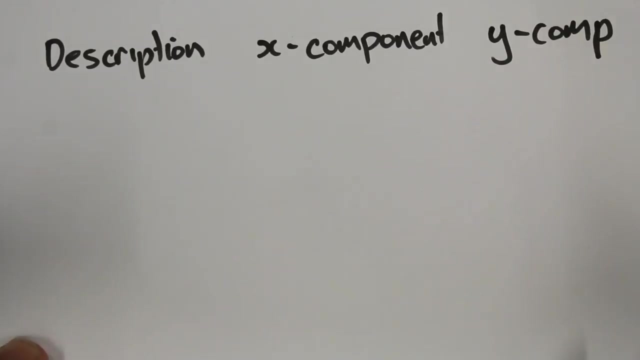 the x component and also the y component. Alright, so the description would be: we have those three forces there and we'll write them. I'm just going to write them down here, So I'll just move this up. Our first force was a 10. 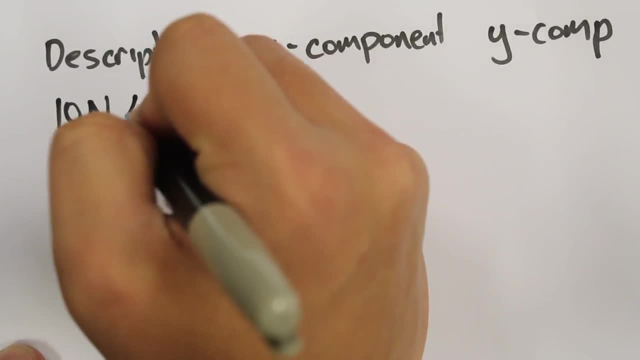 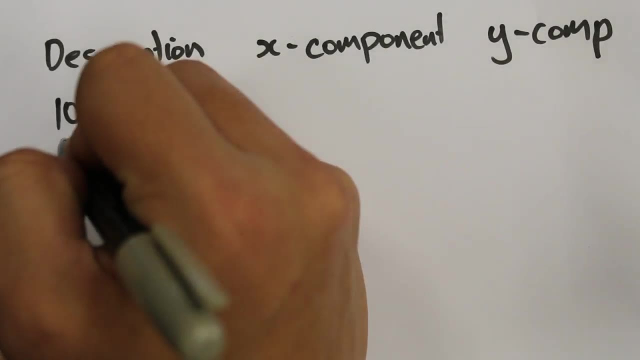 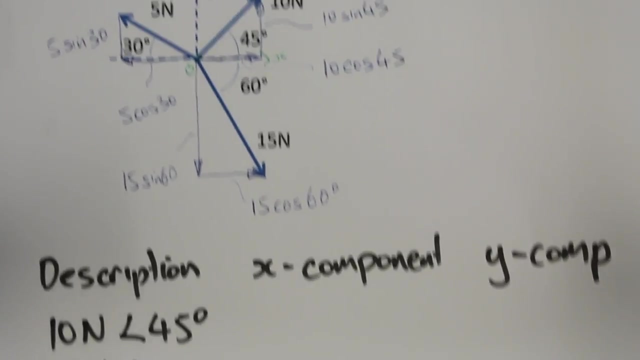 Newton force. It was acting at an angle of 45 degrees as measured from the x-axis. We also have a 5 Newton force which was acting at an angle of 150 degrees. So if we look here, the angle measurement from here to this point here will be: 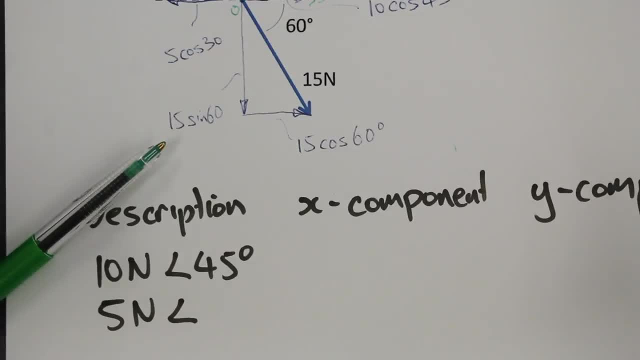 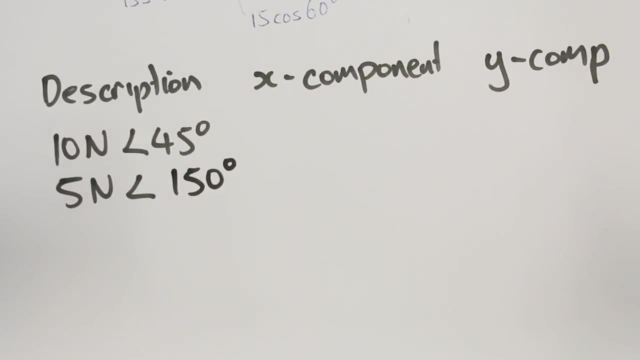 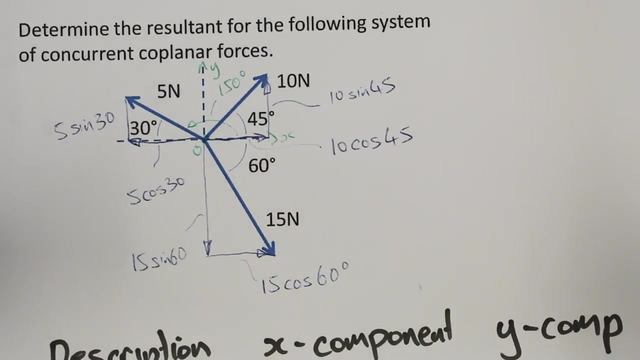 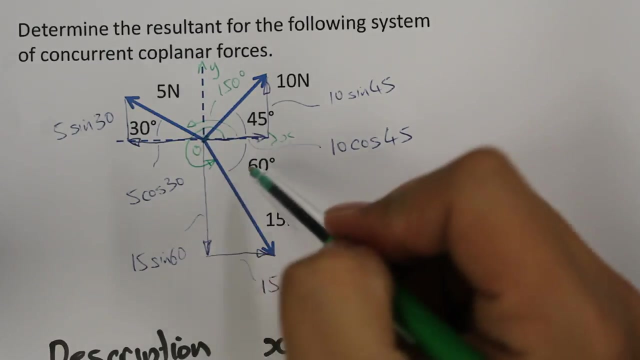 150 degrees. So here our measure is 150 degrees, Same for our 15 Newton force. So if we look at this again, the measure of angle going from the x-axis all the way around to our vector, there will be 360 minus 60 or 300. 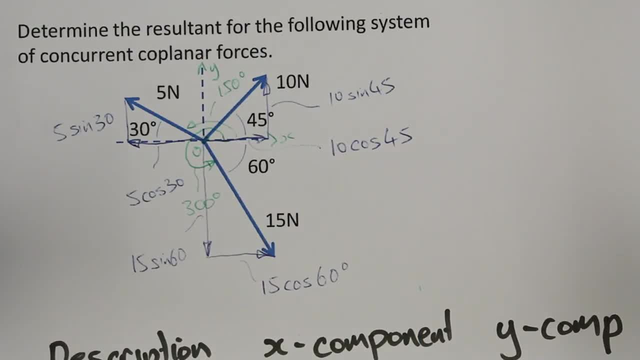 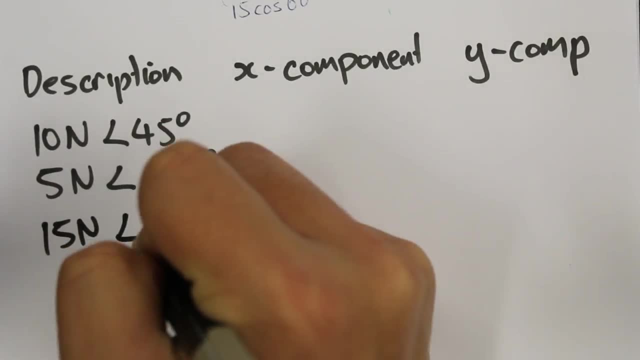 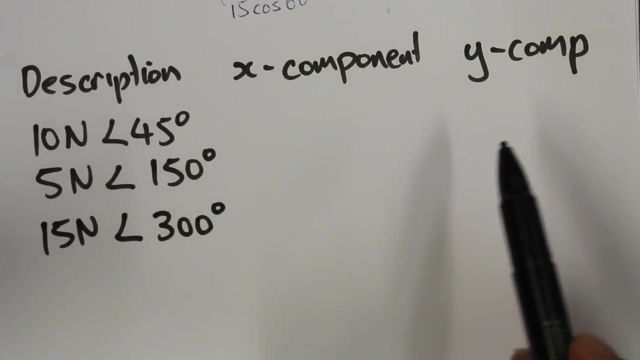 degrees. So let's write that component down. So the 15 Newton force is at an angle of 300 degrees. Alright, so we can write down the x-component and y-component for each force, as long as we measure the angle as measured from the x-axis. 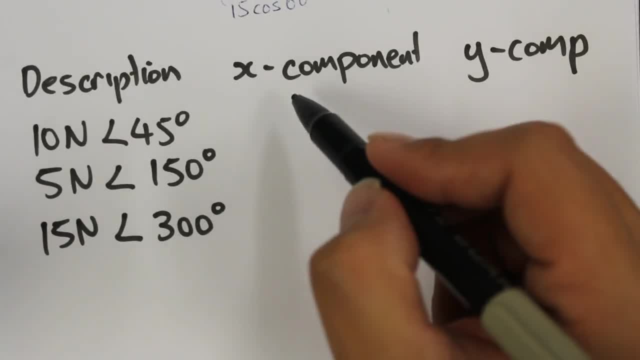 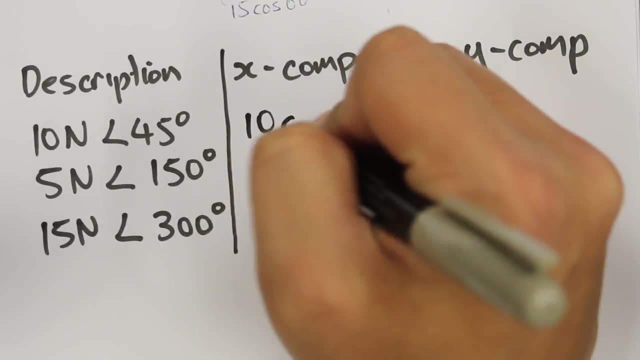 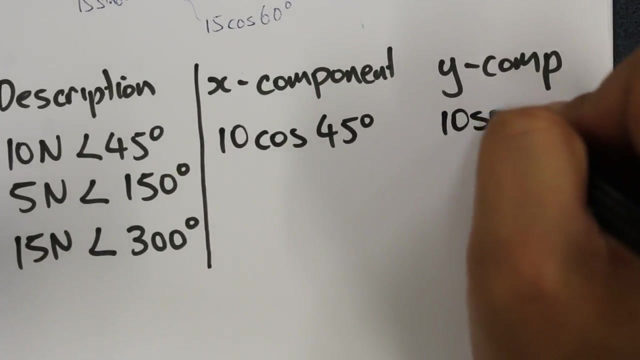 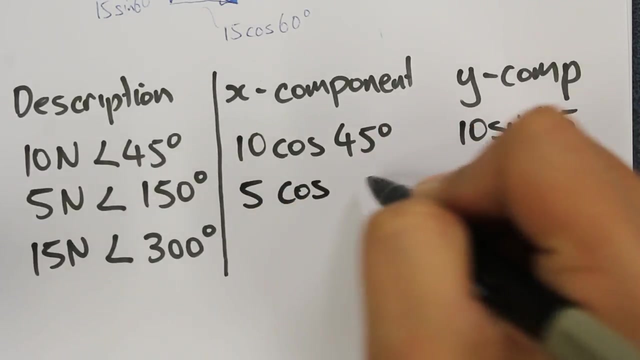 So here we can write down our x-component. So this will become 10 cosine 45, and the y-component would become 10 sine 45.. For the 5 Newton force we have 5 cosine 150, using the angle measured from the x-axis and 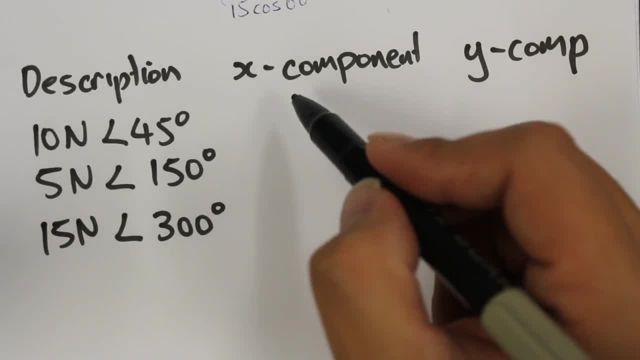 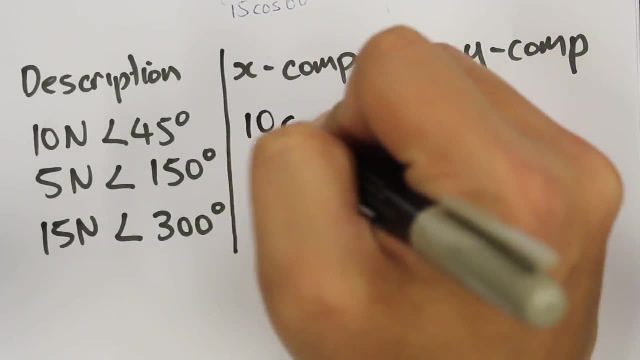 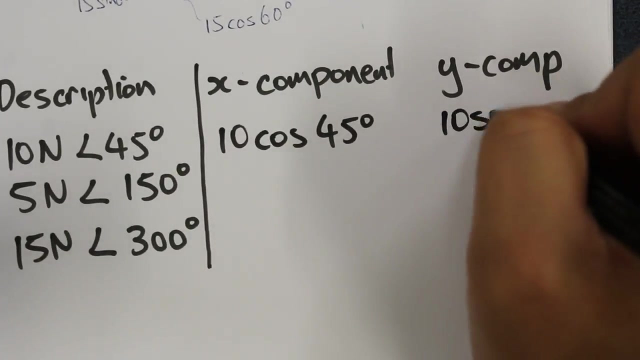 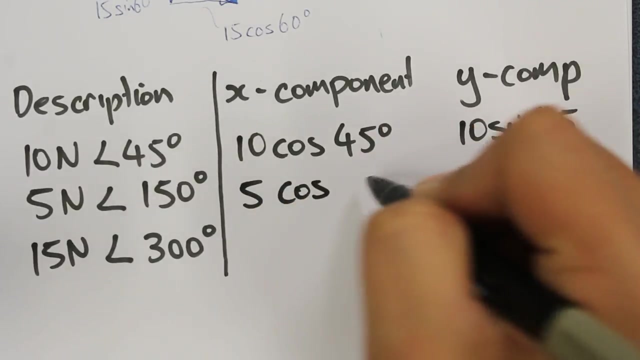 the x-axis. So here we can write down our x components. So this will become 10 cosine 45 and the y component would become 10 sine 45.. For the 5 Newton force we have 5 cosine 150, using the angle measured from the x-axis, and we: 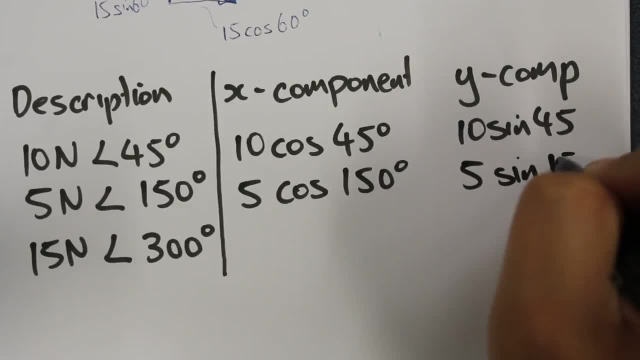 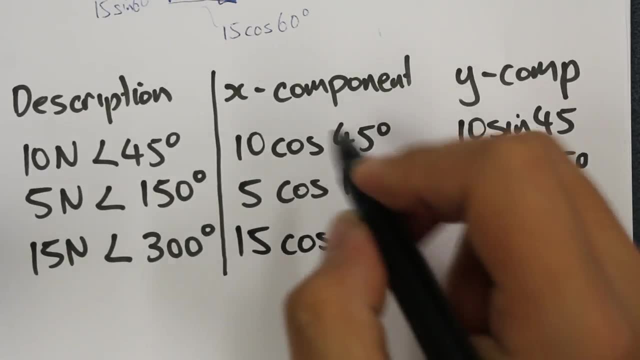 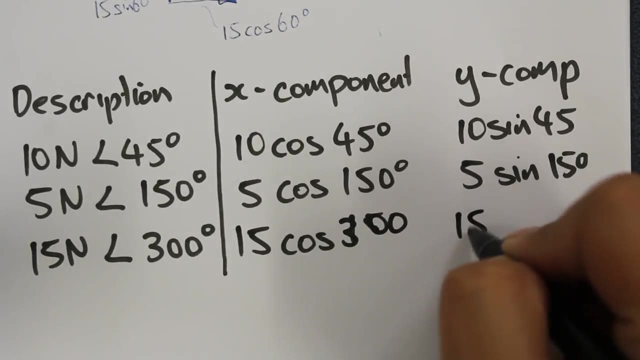 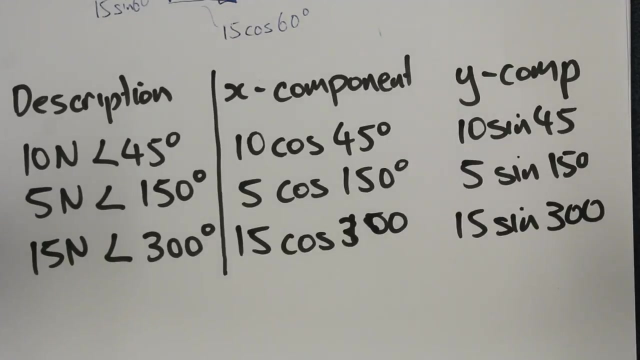 have 5 sine 150. Also for the 15 Newton. so we have 15 cosine 300- sorry, 300- and 15 sine 300.. Alright, so we can now find the total sum of the x components, and that will just be equal to the sum of these three values added together. So we'll go. 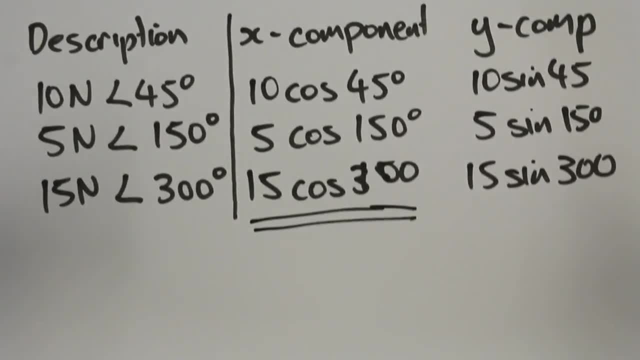 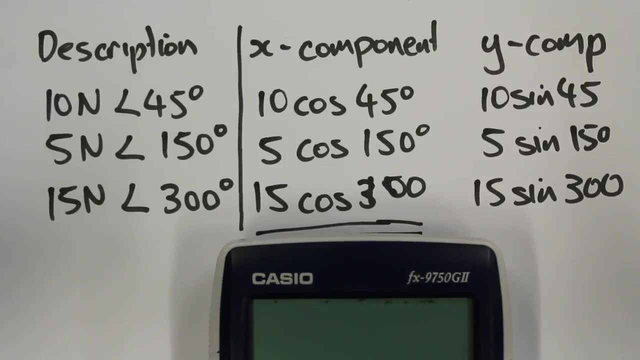 through that summation now. Okay, so here on my calculator I'll type those values in: So 10 times cosine 45 plus 5 times cosine 150 plus 15 times cosine 300.. So you should see that there. I'll press the equals button and we get ten point to four as our total x. 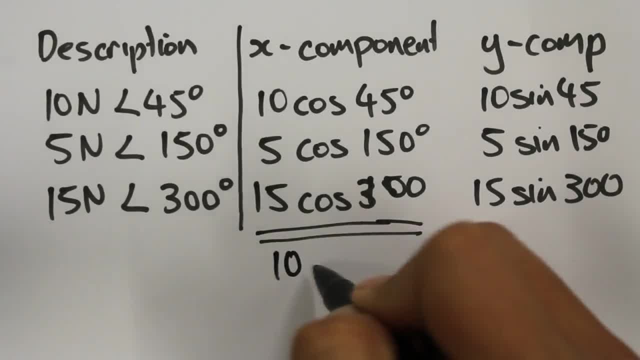 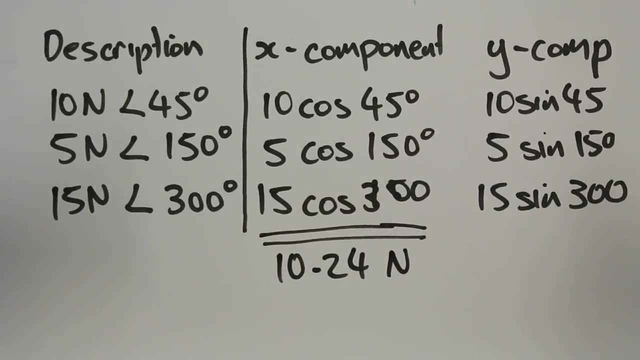 component of our force. the units for this will be Newton's. Okay, so next we can do the same thing for the y- sorry, x- component. So we're gonna just simply add this up like this: gets10.24, and then thisเม: 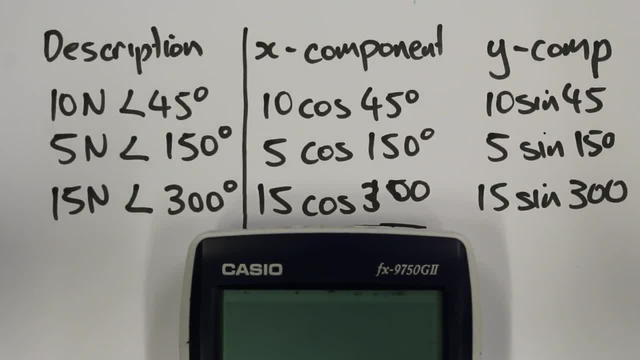 same thing for the y component of force. So for the y components we have 10 times sine 45 plus 5 times sine 150 plus 15 times sine 300.. Press the execute button and here we get minus 3.42 rounded for our value of force, The units being: 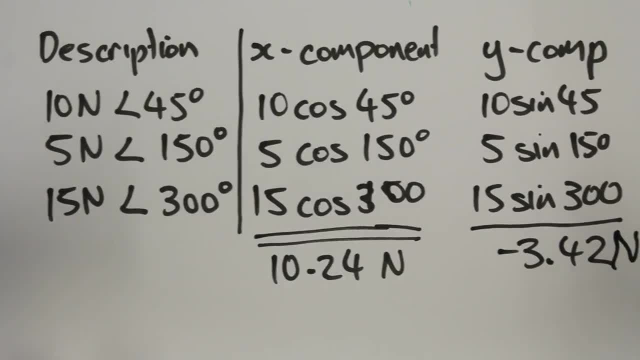 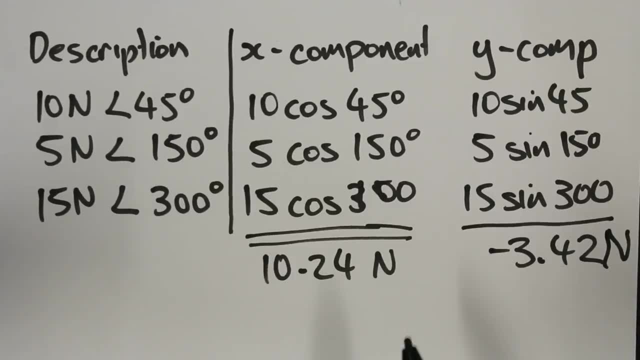 Newtons as well. Okay, so now we've got the x component and the y component of our resultant force. This would be the combined effect of those three forces acting on our system. Next step is to now draw a diagram showing these forces, So we'll move to. 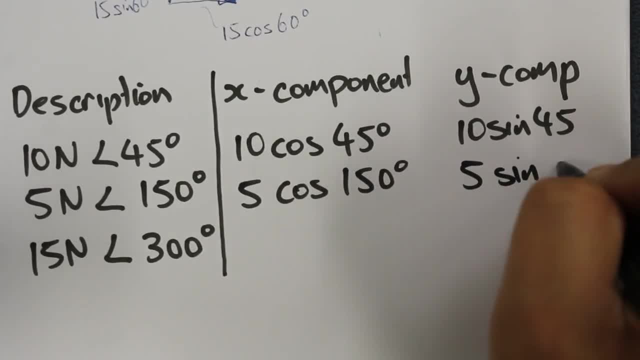 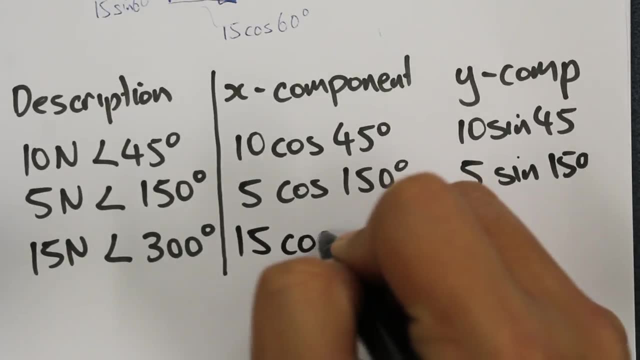 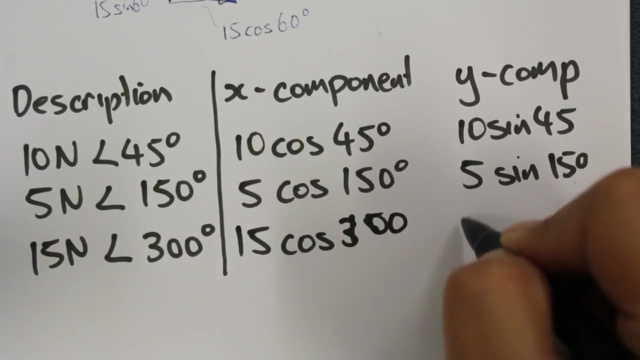 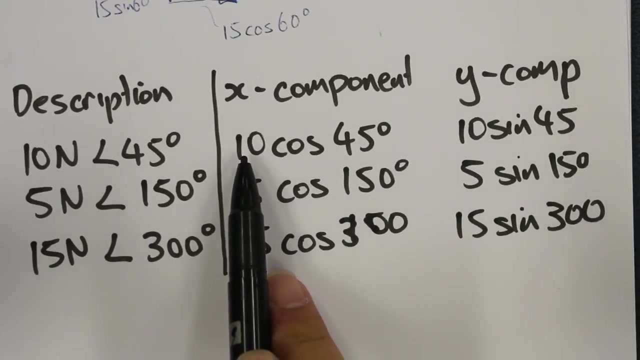 we have 5 sine 150. Also for the 15 newton. so we have 15 cosine 300- sorry, 300- and 15 sine 300.. Alright, so we can now find the total sum of the X components, and that will just be equal to the sum of these three values added. 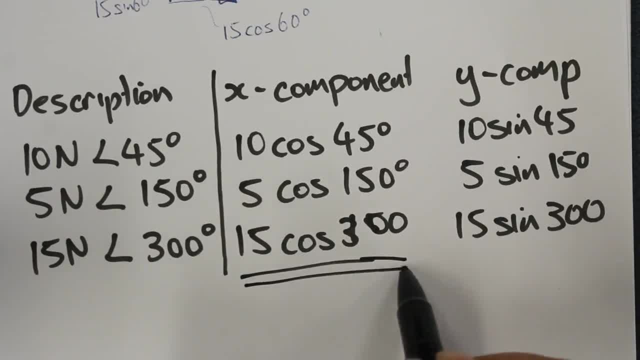 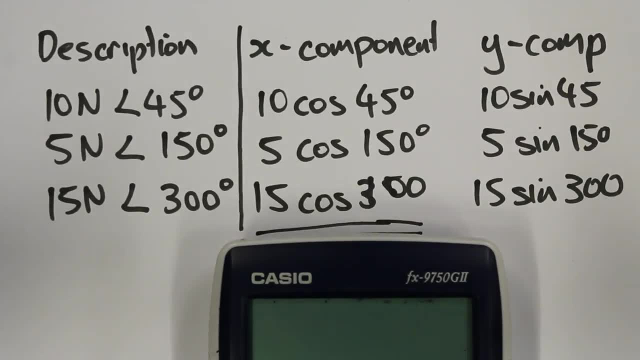 together. So we'll go through that summation now. Okay, so here on my calculator I'll type those values in: so 10 times cosine 45 plus 5 times cosine 150 plus 15 times cosine 300.. So you should see that there. I'll press the equals button and we 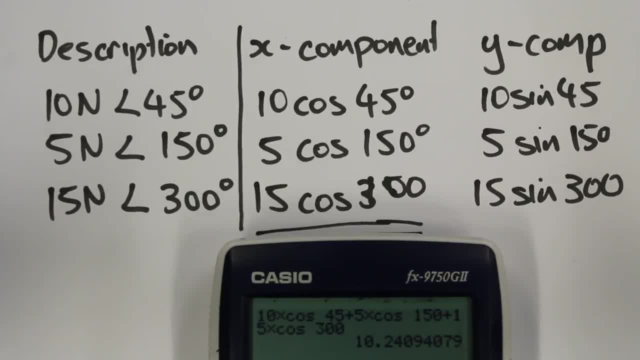 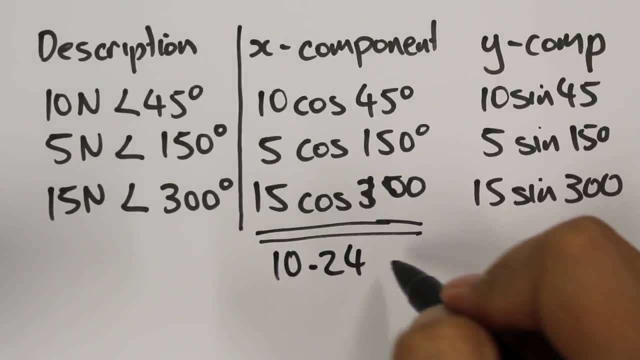 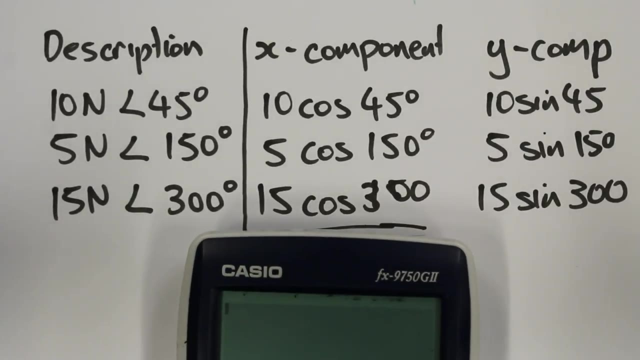 get 10.24 as our total X component of our force. The units for this will be Newtons. Okay, so next we can do the same thing for the Y component of force. So for the Y components we have 10 times sine 45 plus 5 times sine 150 plus 15 times sine 300. 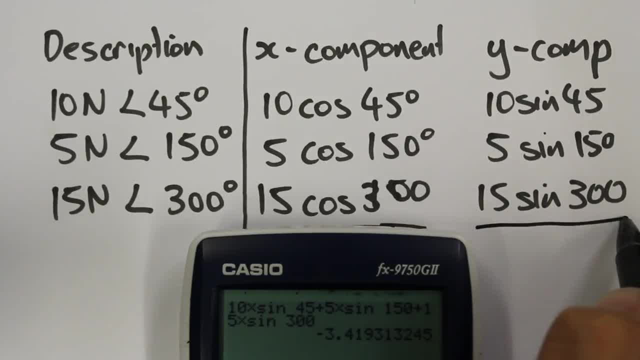 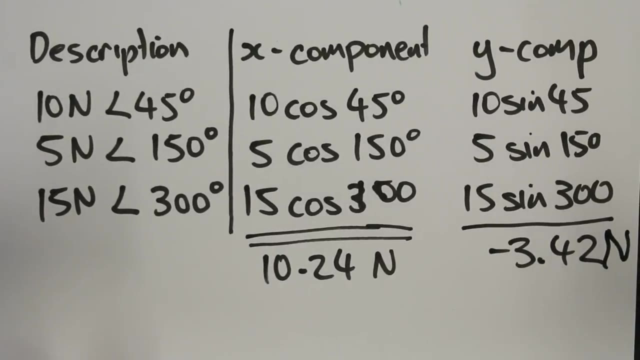 Press the execute button, and here we get minus three point four, two rounded for our value of force, the units being Newtons as well. Okay, so now we're. Now we've got the x component and the y component of our resultant force. This would be the combined effect of those three forces acting on our system. 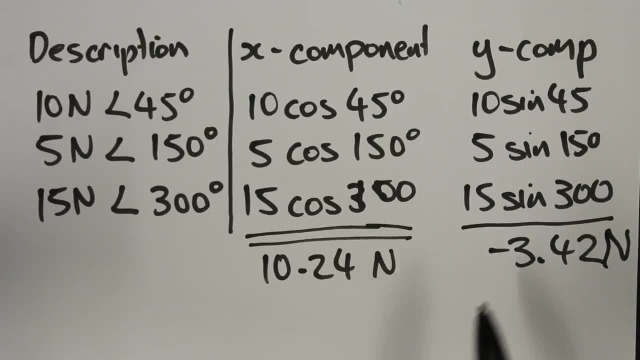 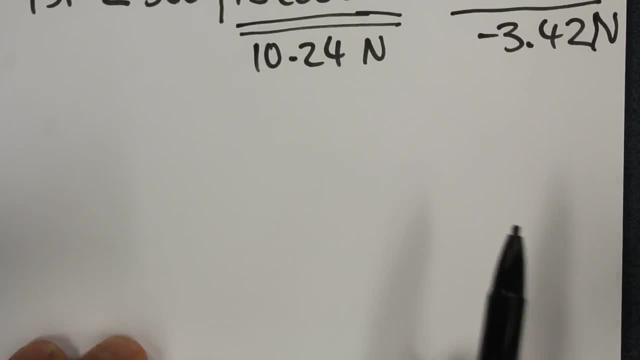 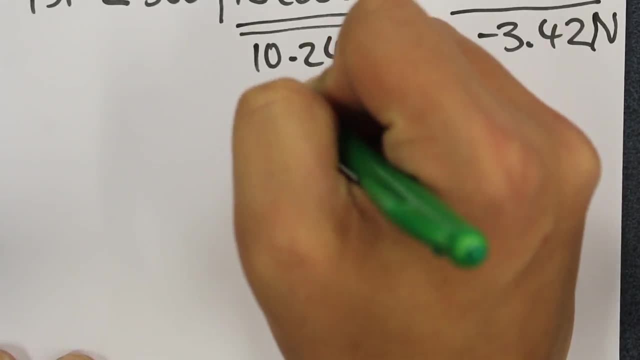 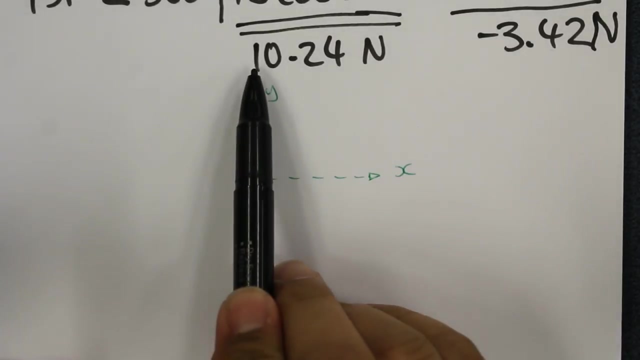 Next step is to now draw a diagram showing these forces. so we'll move to that step now. So we'll indicate the y direction. so this is y and this is the x direction. Here we see our x component is 10.24 and it's positive. so it goes towards the right hand side. 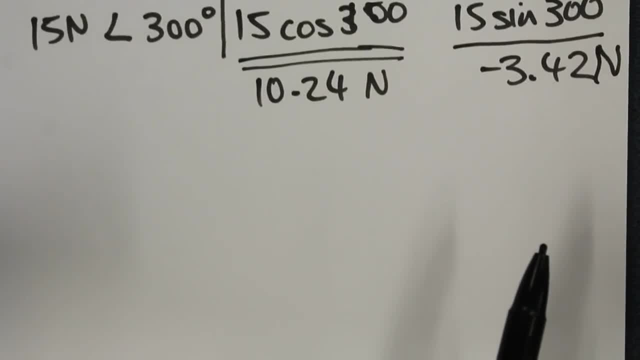 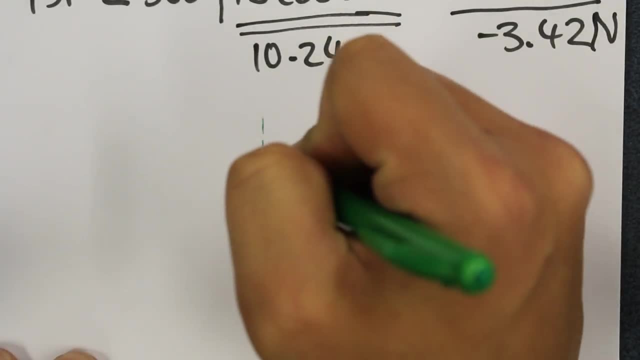 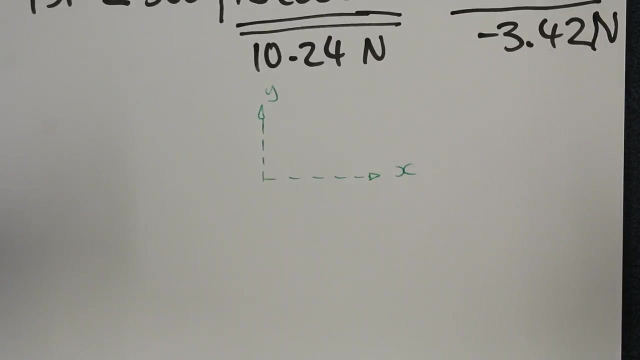 that step now. Okay, so move up. Okay, so we'll indicate the y direction. So this is y and this is the x direction. Here we see our x component is 10.24 and it's positive, So it goes towards the right hand. 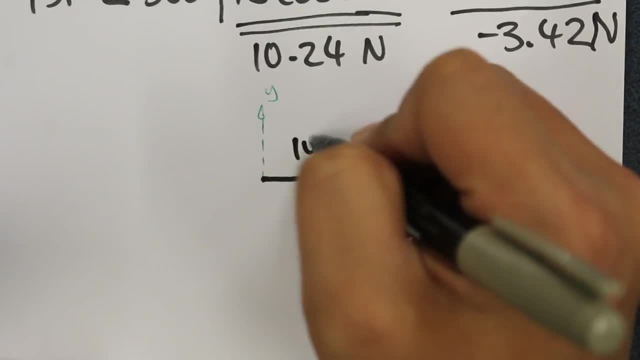 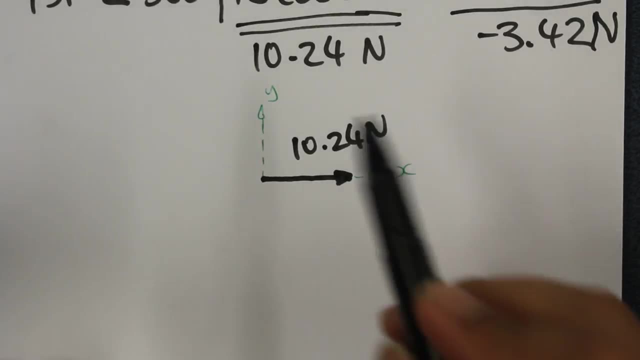 direction. So it goes towards the right hand direction. So it goes towards the right hand side, towards the positive x-axis as 10.24 Newtons For the y component. it's negative, So it moves in the negative y, So that's a positive y. 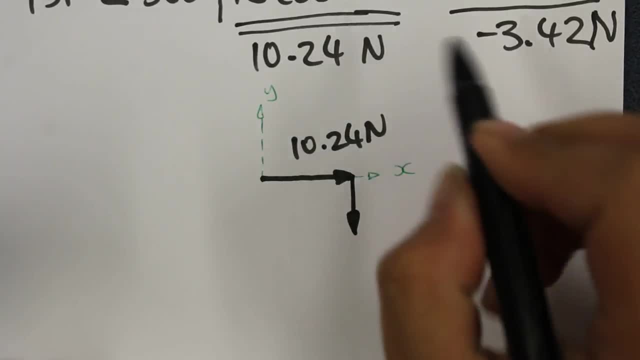 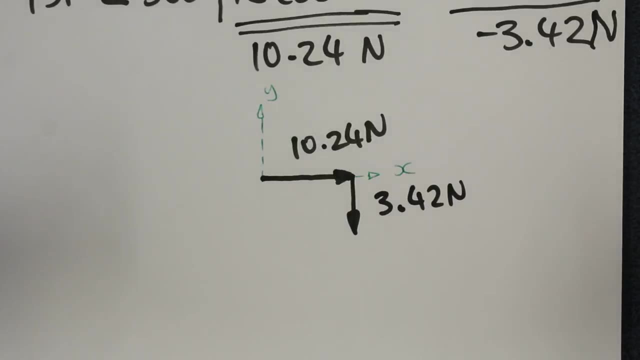 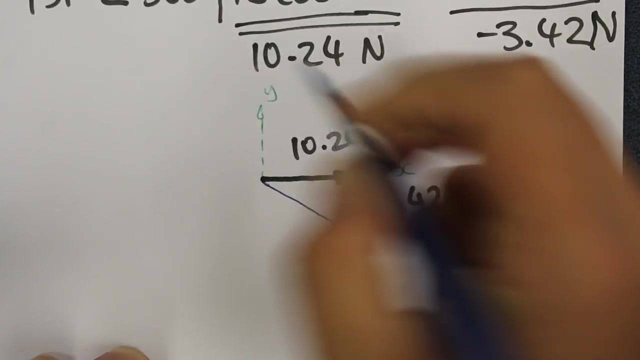 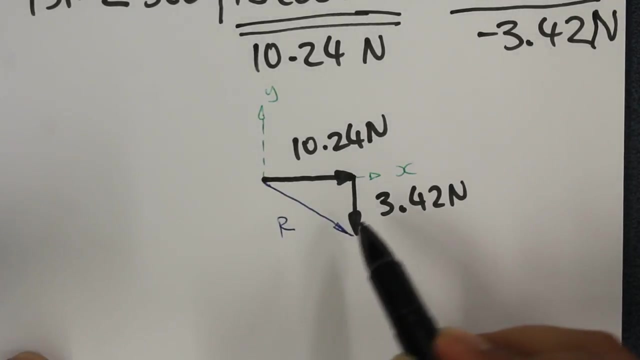 negative going down. This goes down, The value that it goes down is 3.42 Newtons, And our resultant force will be the force that connects these two vectors together. So this one here Call that r. Okay, so our resultant force r, and we can find that out using 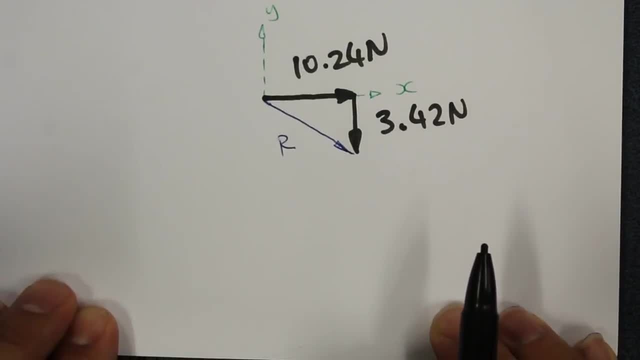 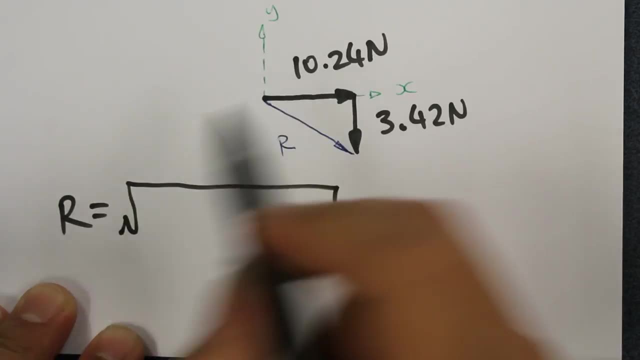 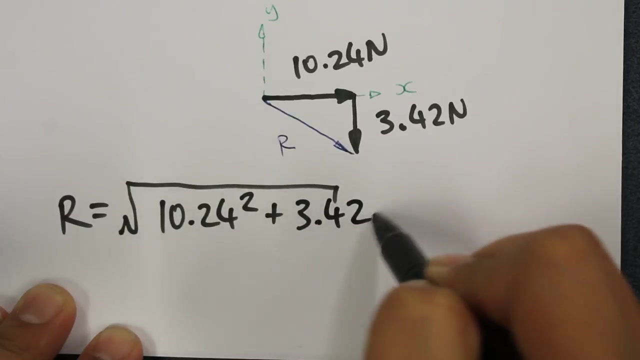 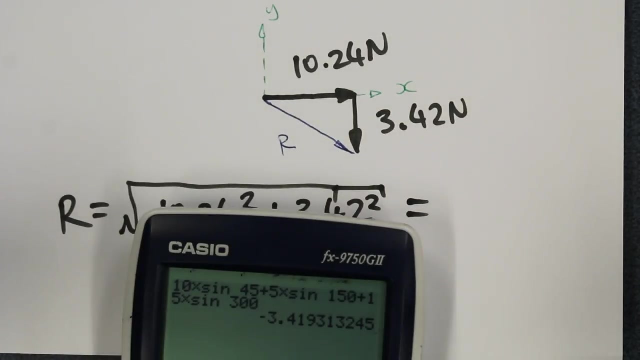 Pythagoras. So, moving that up, R will be equal to the square root of 10.24 squared plus 3.42 squared. The value that we get here will be equal to alpha square root of alpha a squared plus alpha b squared, and in brackets we get 10.79, or around about 10.8, as our value for our. 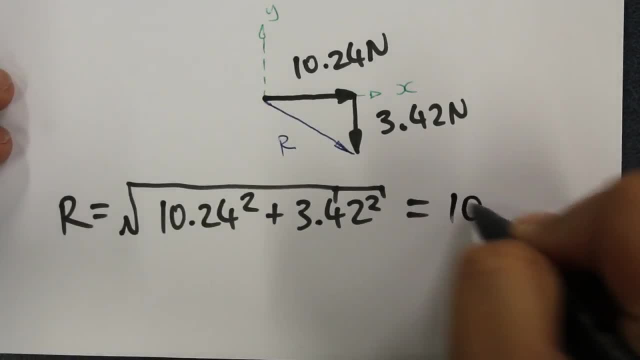 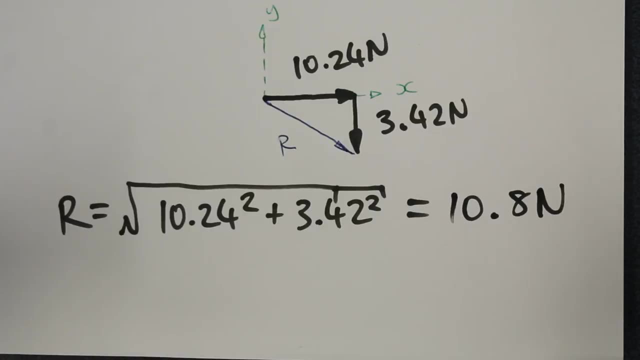 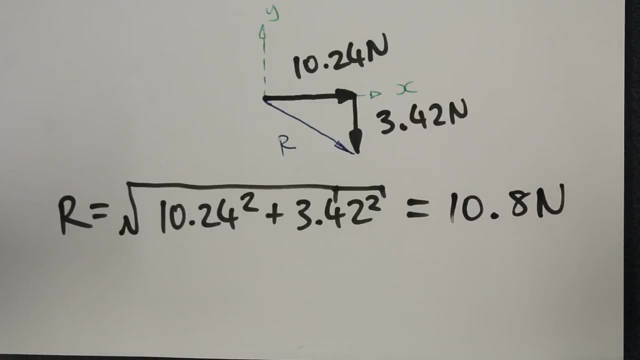 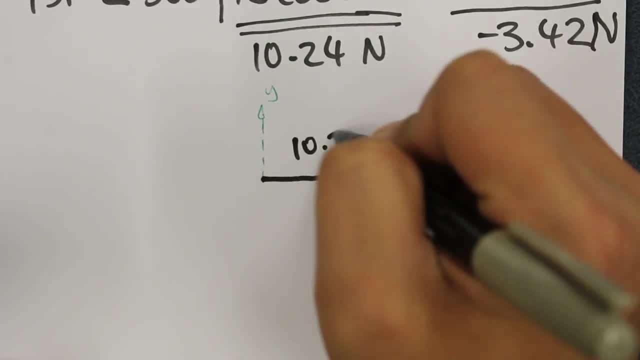 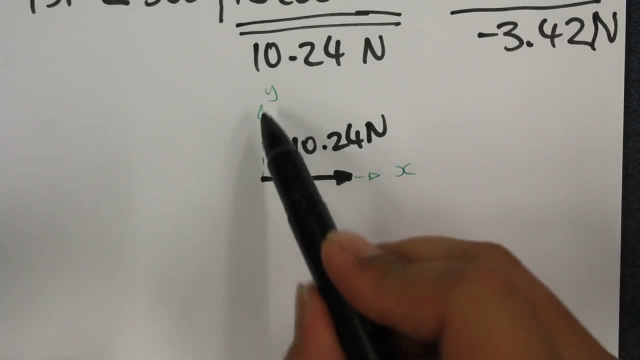 towards the positive x axis as 10.24 newtons. For the last step, we're going to draw a diagram showing these forces acting on our system. Here we see our y component. it's negative, so it moves in the negative y. 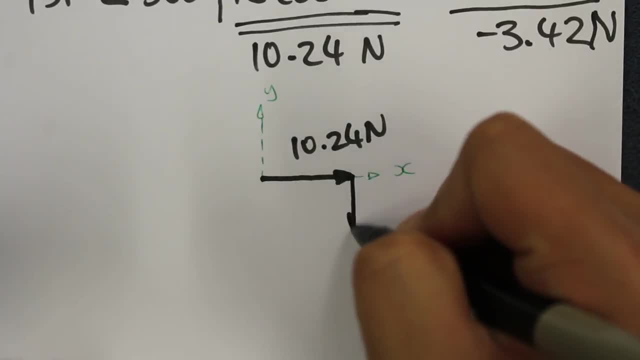 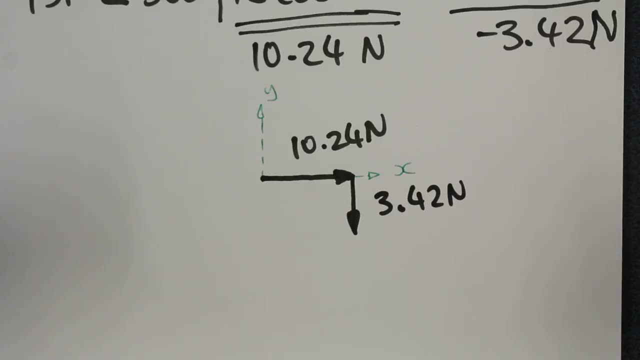 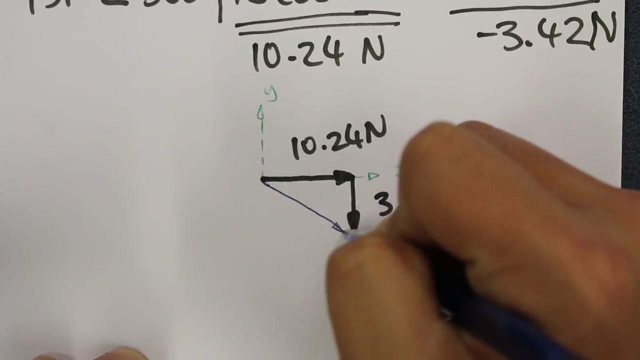 so that's the positive, y negative going down. this goes down. The value that it goes down is 3.42 newtons And our resultant force will be the force that connects these two vectors together. so this one here, call that R. 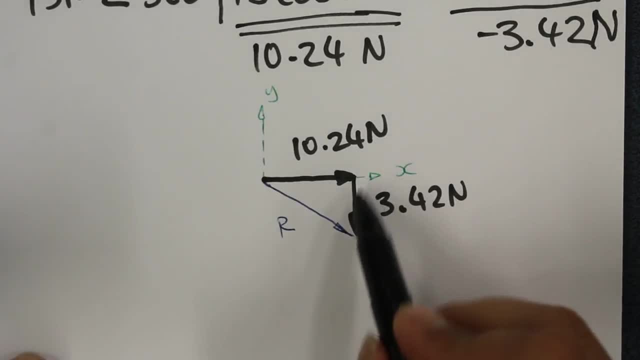 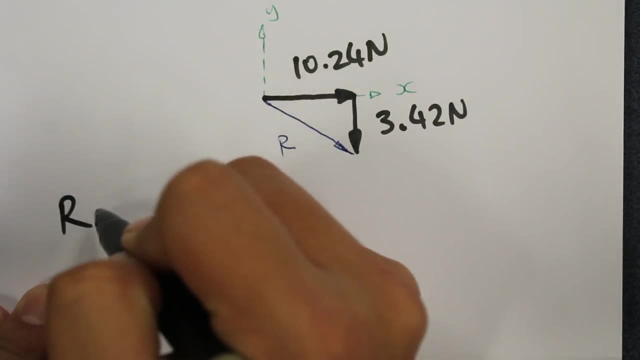 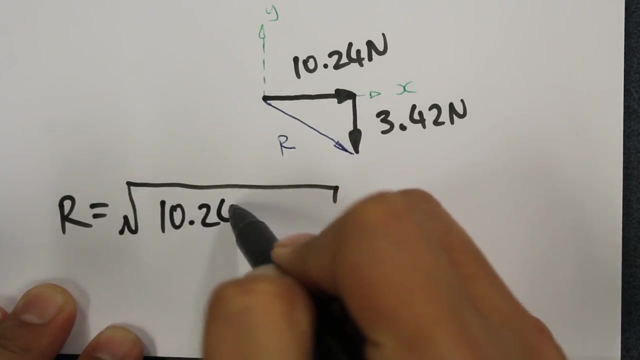 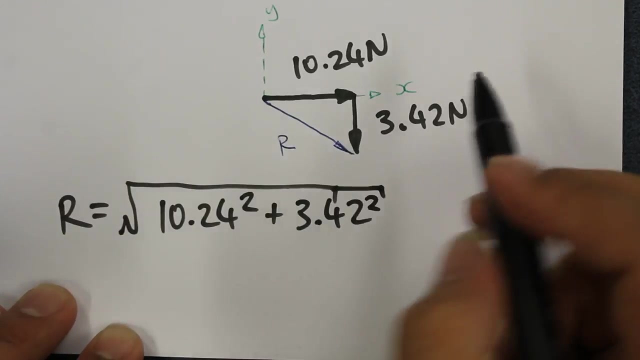 Okay so our resultant force R: we can find that out using Pythagoras. Okay so our resultant force R, we can find that out using Pythagoras. So, moving that up, R will be equal to the square root of 10.24 squared plus 3.42 squared. 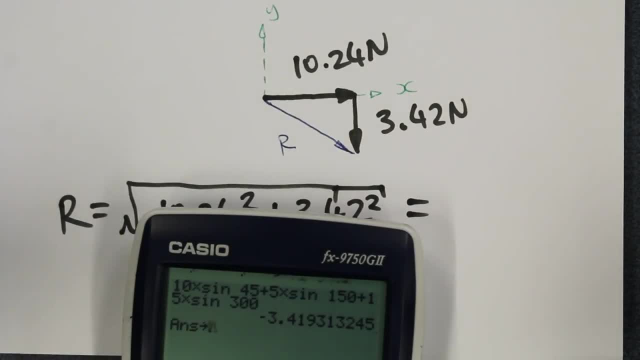 The value that we get here will be equal to go alpha square root. the value that we get here will be equal to go alpha square root of alpha a squared plus alpha b squared, and in brackets we get 10.79, or round about 10.8 as our value for our resultant force. 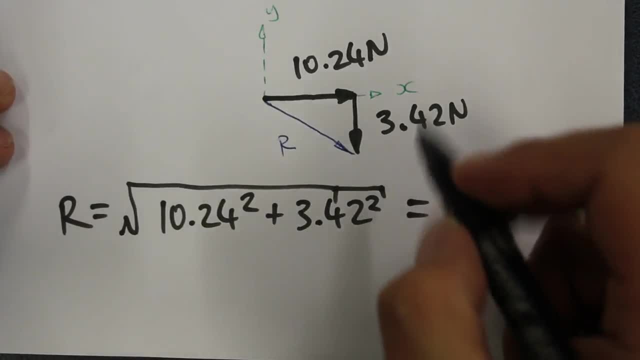 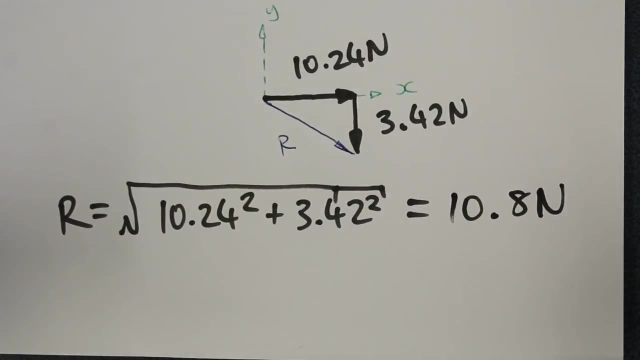 we get 10.79, or round about 10.8 as our value for our resultant force. So 10.8 newtons as our resultant force, So 10.8 newtons as our resultant force. So we also need to find the angle at which this force acts. 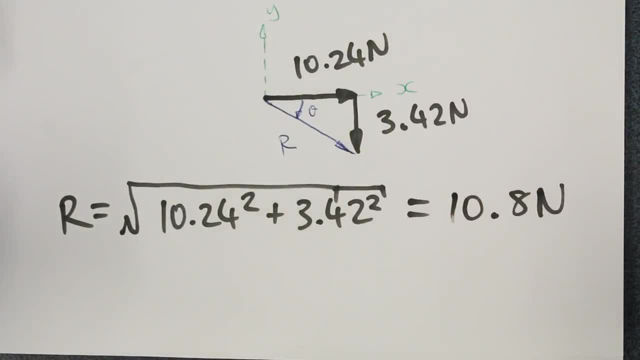 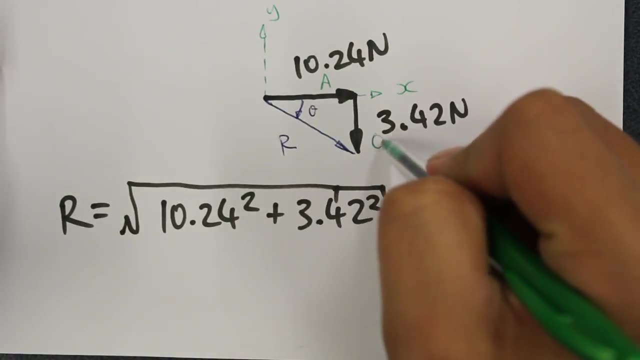 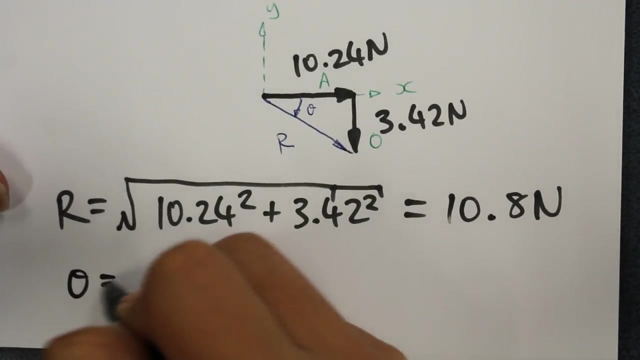 So that's this angle here, theta. Now, recalling from your basic trick, this would become the adjacent side and the opposite side. So we can find the angle theta by using the tan rule. So theta is equal to the inverse tan of the opposite divided by the adjacent side.